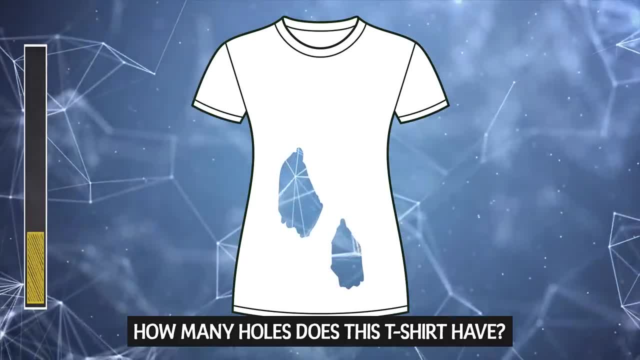 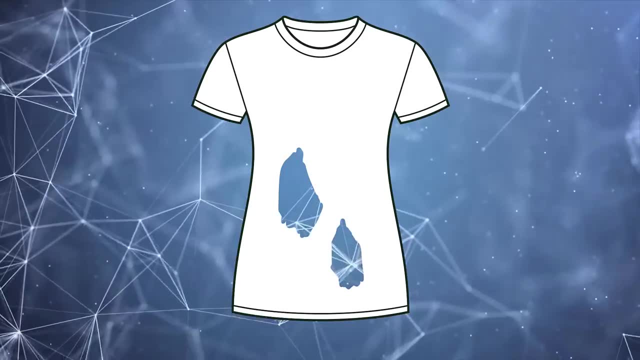 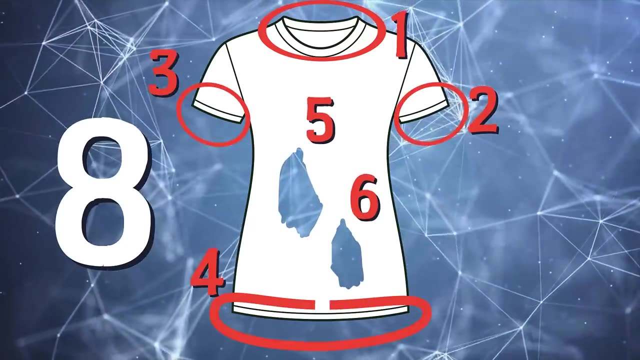 Don't ever go to the hospital again. Now that this question doesn't specify which holes exactly, So the right answer is 8.. They are the neckline, two sleeves, the bottom of the T-shirt and 4 holes in the middle. 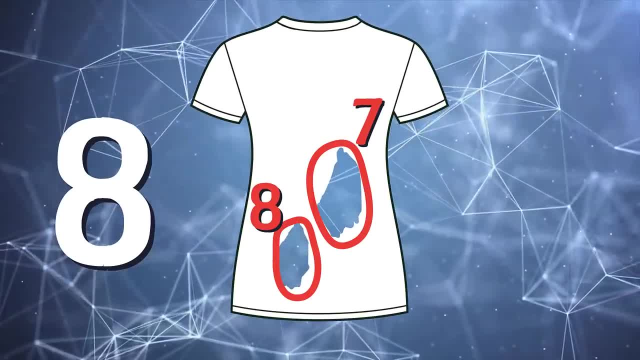 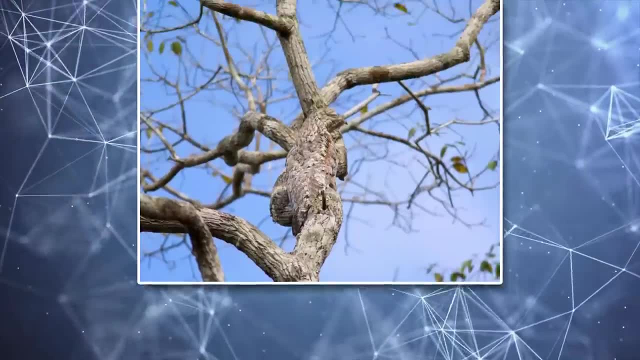 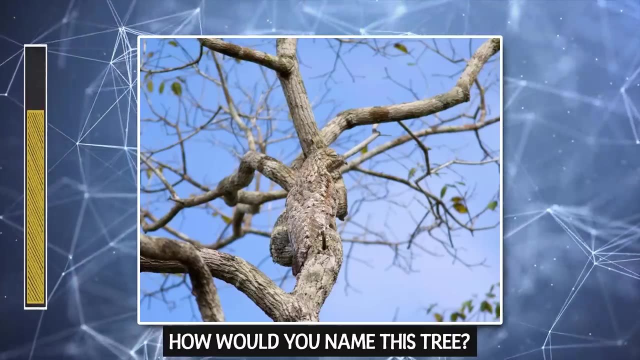 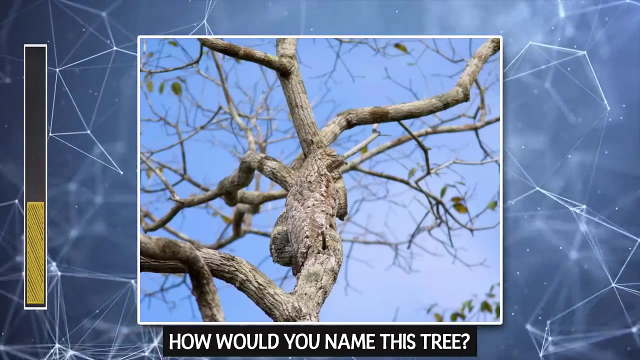 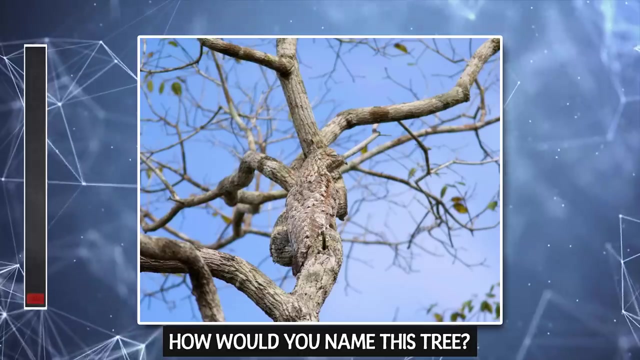 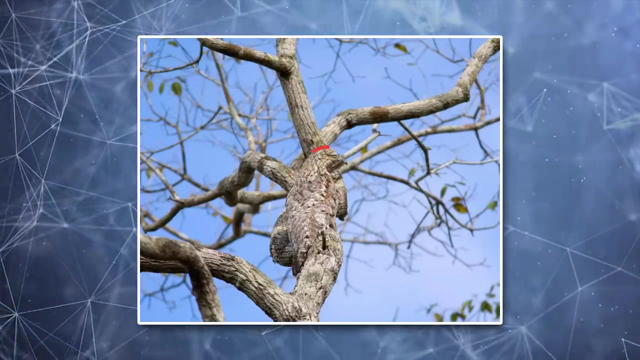 Two in the front and two in the back, because we can see the background through them. 5.. How would you name this tree? Write the names that came to your mind in the comment section below. But the actual challenge was to notice the camouflaged bird on the tree. 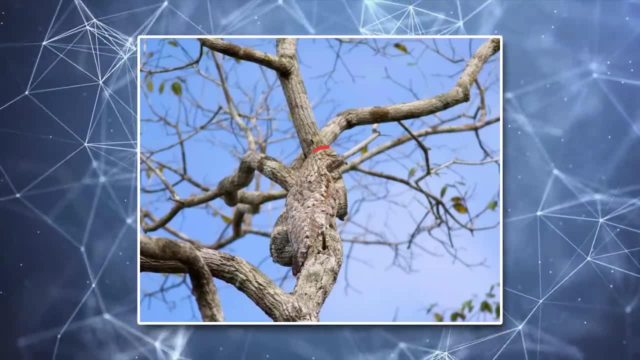 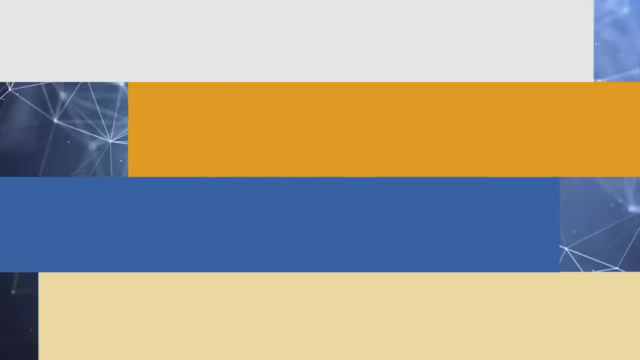 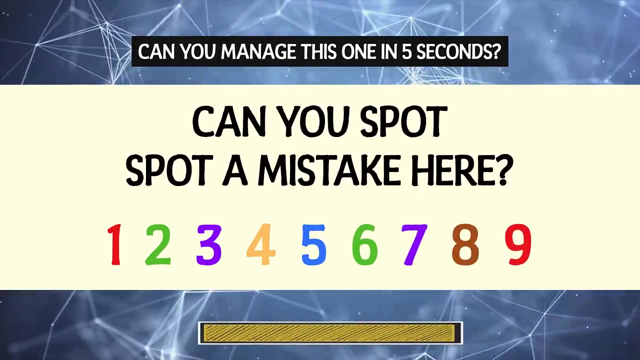 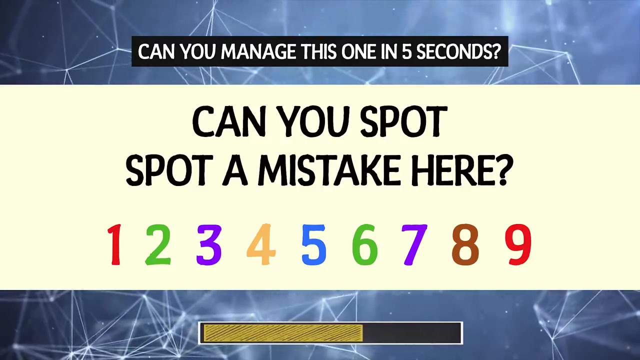 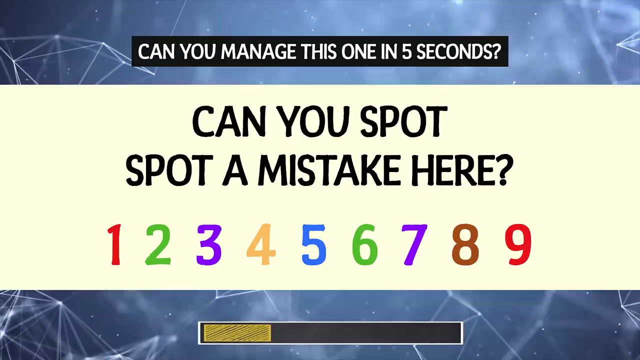 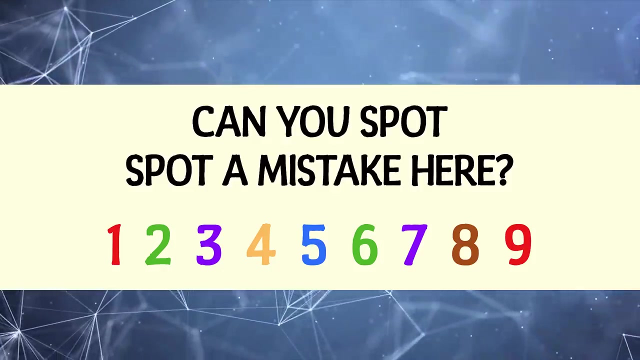 If you did, well done. 4. Can you manage this one in 5 seconds? I'll give you 20 seconds, but try to solve it as fast as possible. 5. How would you name this tree? The mistake is not in the numbers or their colors. The mistake is that the word 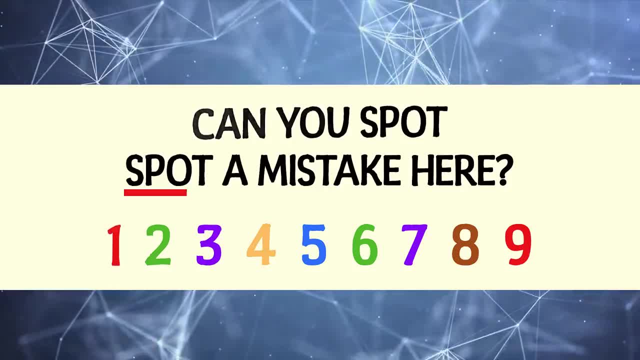 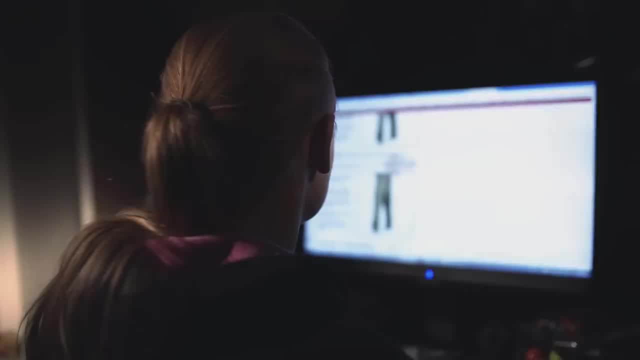 spot appears twice. Your brain doesn't always show you the reality. It often shows what it is used to. There are many short texts on the internet that have repeating words that most people don't notice until they finish the text and read the description. 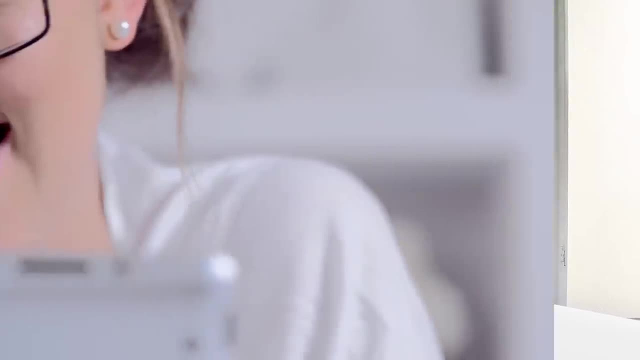 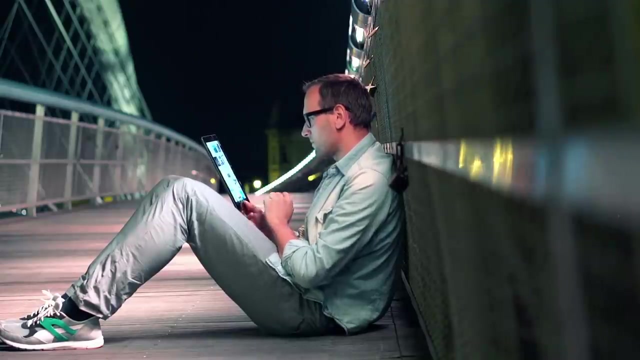 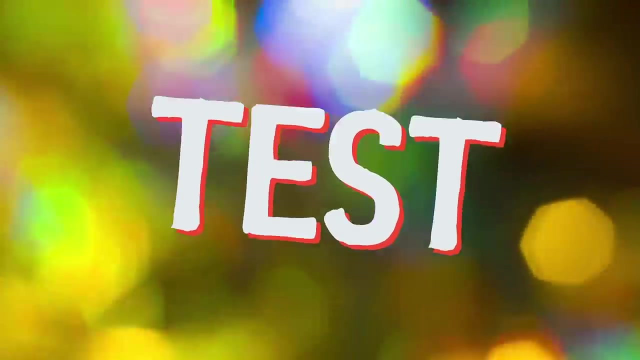 If you have bad eyes, you might have noticed that things you couldn't see from a distance become clearer when somebody tells you what's written there. It's not that your eyes became better, It's your brain completes the picture. 3. Do you see a hidden baby? That's not mine either. 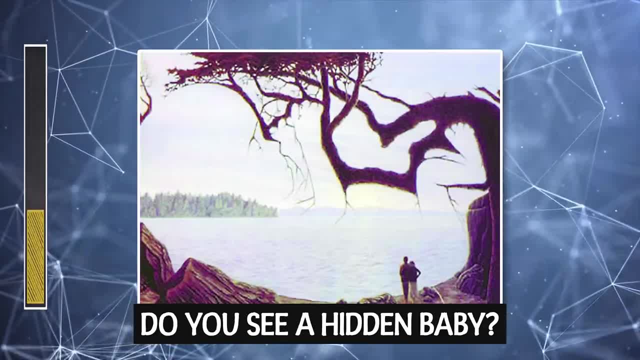 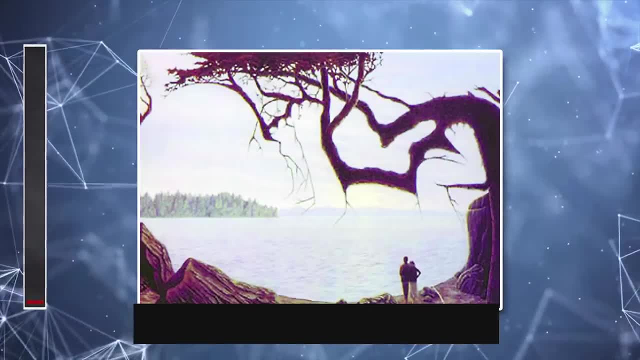 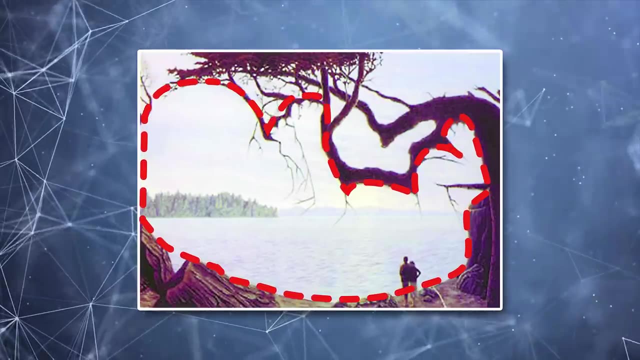 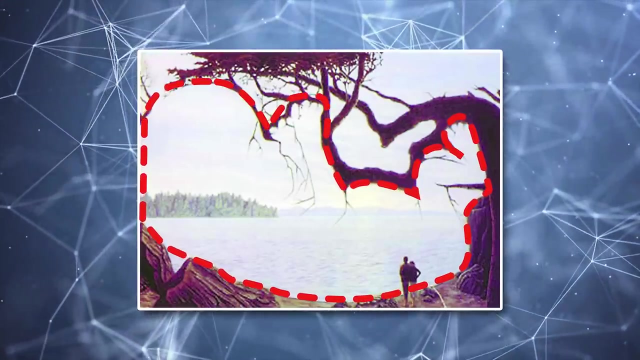 If you follow the thin branches of the tree, you will see the outline of a baby in the fetal position. Its feet and toes are on the right side of the picture, arms are in the middle and head is on the left. One more thing: It's good that he doesn't have teeth, because his bark is better than his bite. 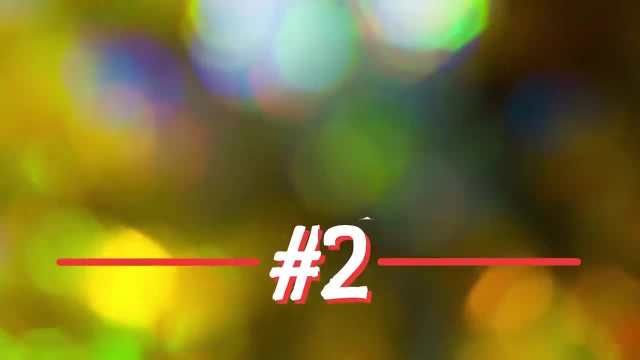 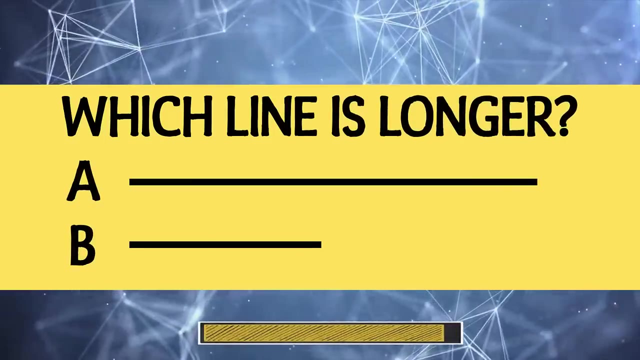 5. How would you name this tree? What word of the day would be correct at this time? Write comments on whatever points you want to, as I will chat with you. Test Nr 2.. Which line is longer? 7. Which of these lines does Stonewall say? 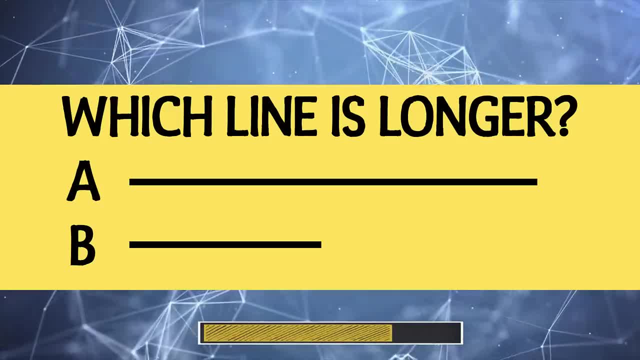 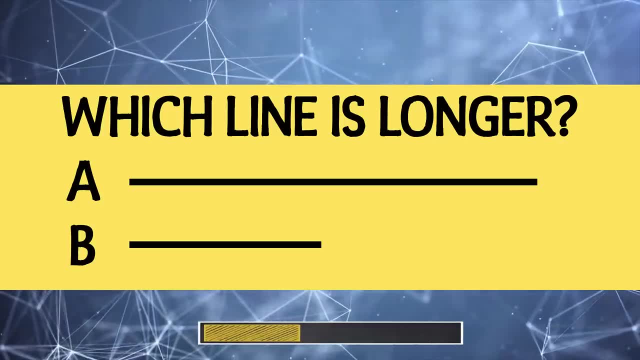 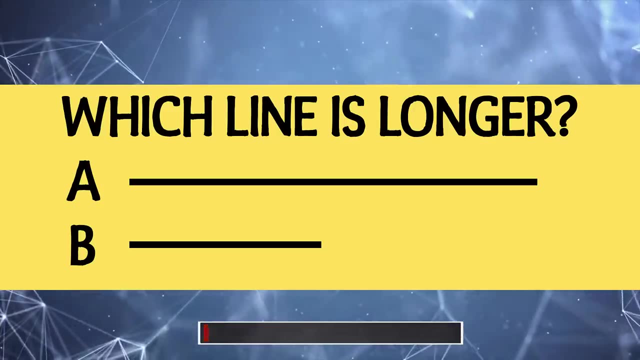 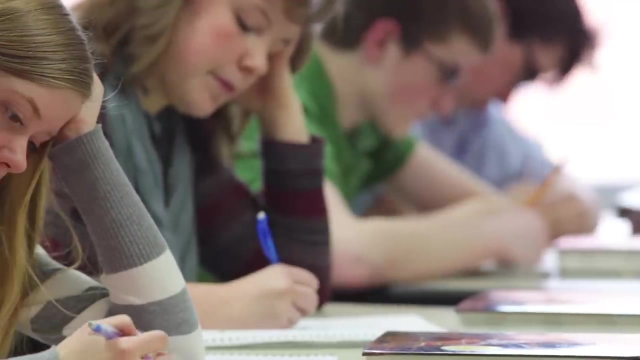 8. Which line gives more points? 9. Which of these lines do you understand? See the videos of many Priest Boyauf English Runs on course. there are 3 better clues. One question: whichwise is the closest Du longer? It's so obvious, right? Well, not for everybody, Or rather not always. 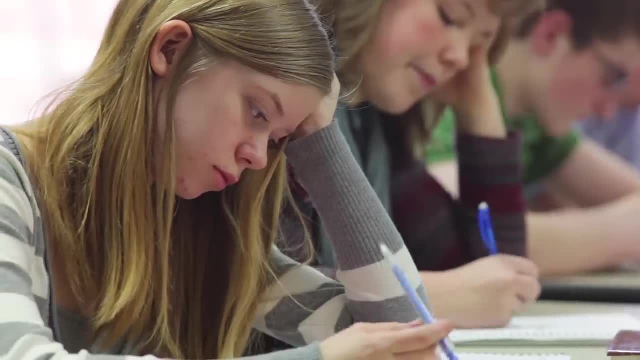 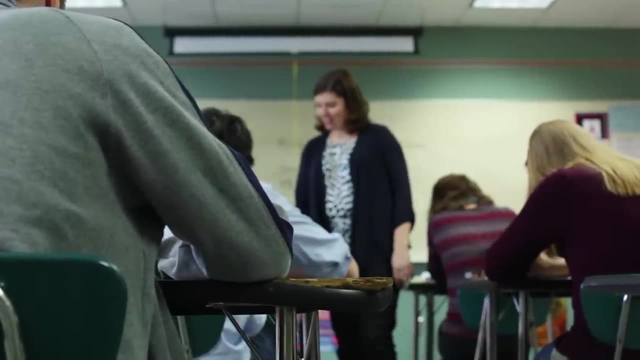 There was a research on conformity that looked like this: Five people were asked which of two lines was longer. The answer was always simple, but four of the tested people were asked to lie, So technically there was only one real subject. The people lied very convincingly. 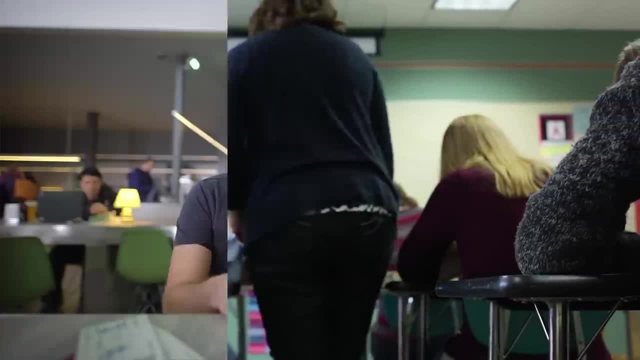 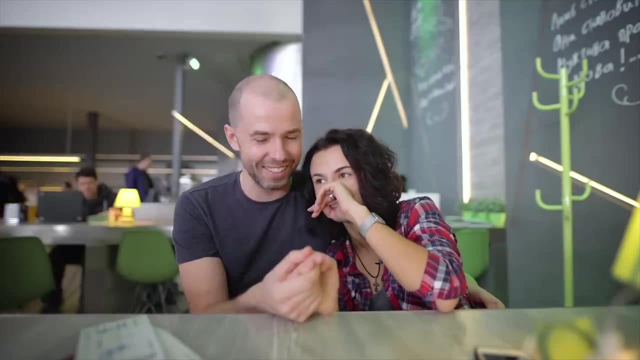 so the subject didn't want to stand out and gave the wrong answer. The same phenomenon can be illustrated with jokes. If you're in a group of people and somebody tells a joke that everybody finds funny, you will laugh too, even if you don't. 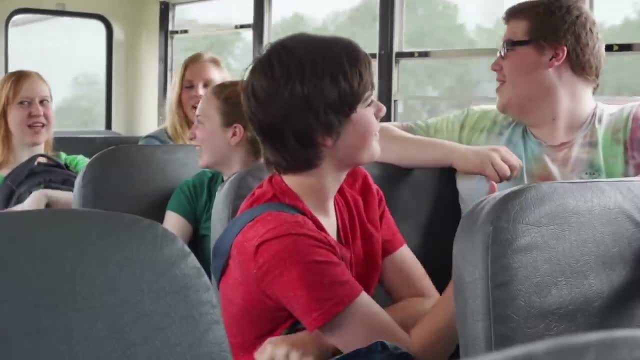 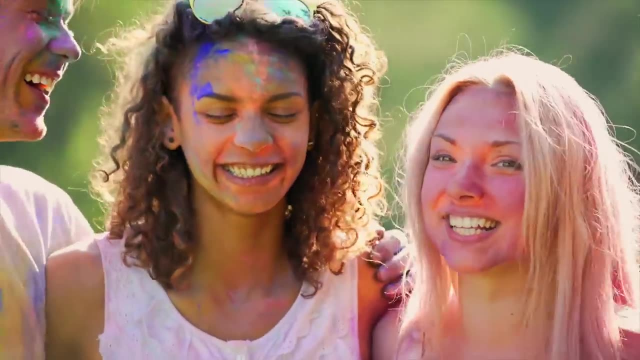 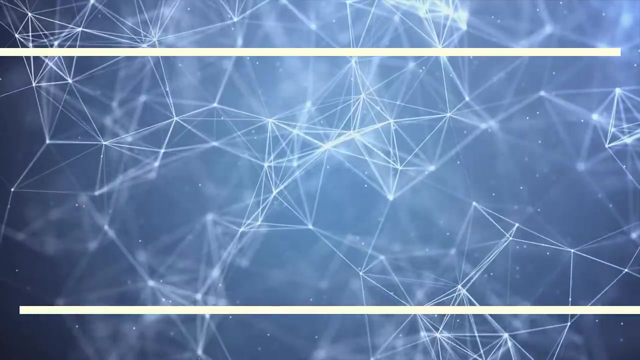 get it or don't think it's funny. Well, maybe not you, but approximately 75% of people do so. Of course, everybody laughs at my jokes, right? Liars Alright. test number one: Can you spot Mike Wazowski? 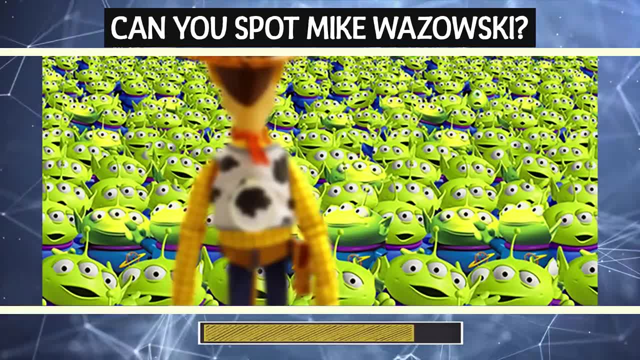 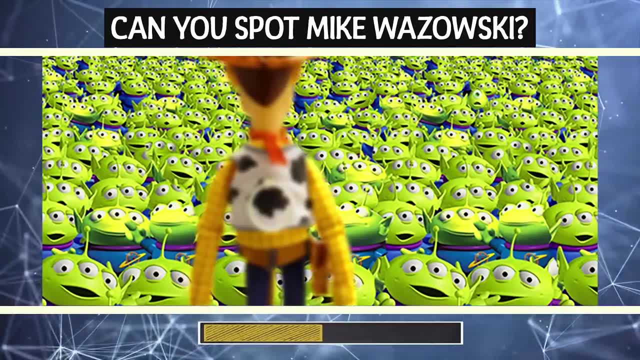 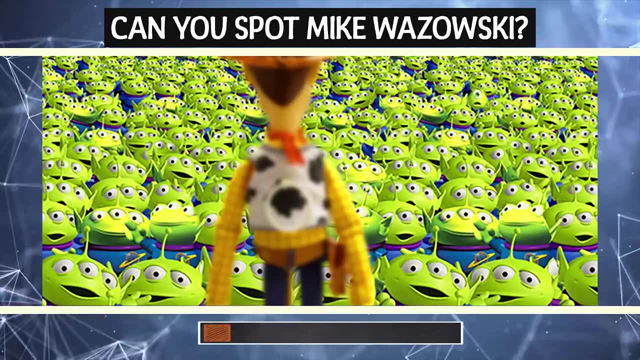 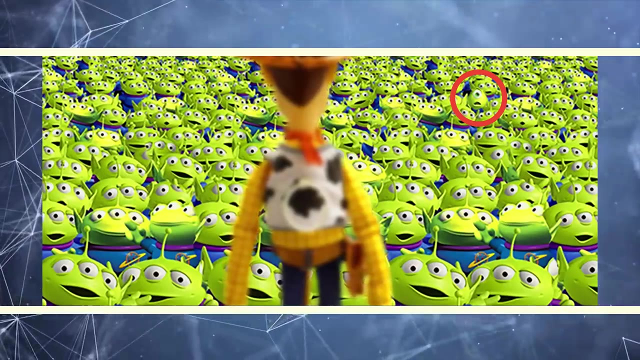 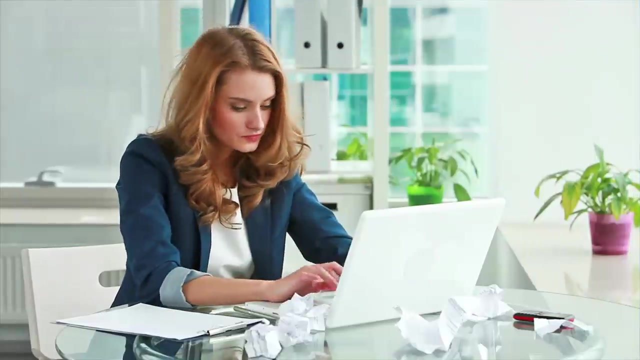 There he is Green, but still very different. Now let's talk about your results. If it took you more than 20 seconds to answer each question or you didn't manage all the tasks, it means that you have the brain of a mature person.